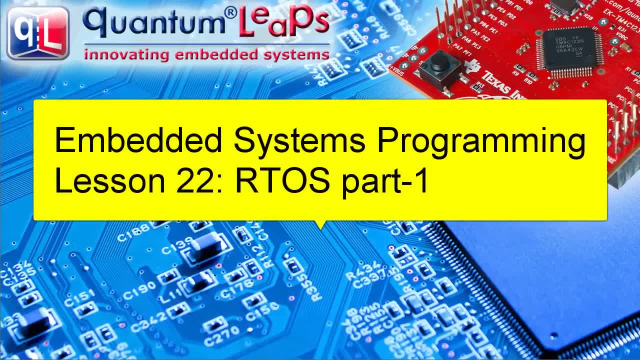 Welcome to the Modern Unbanded Systems programming course. My name is Miro Samek, and in this lesson I'll finally introduce the concept of a real-time operating system, RTOS. At this point let me clarify right away that when I say RTOS, I mean here a real-time kernel. 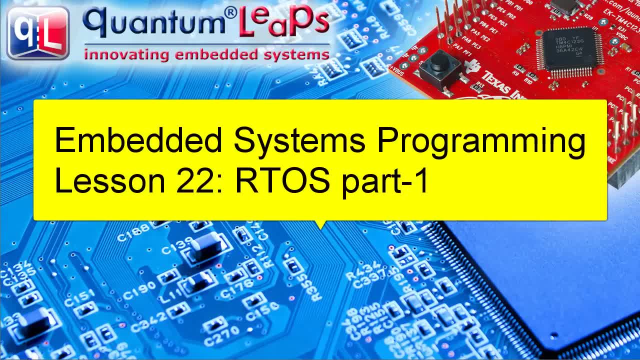 component of the RTOS which is responsible for multitasking. I specifically don't mean here hardware abstraction layers, device drivers, file systems, networking software or other such components sometimes attributed to the RTOS. In this first lesson on RTOS, you will see how to extend the foreground-background architecture. 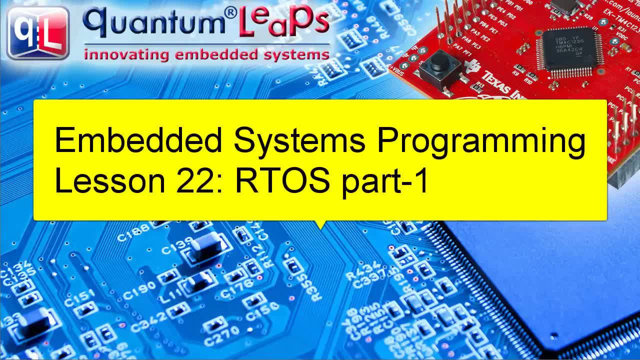 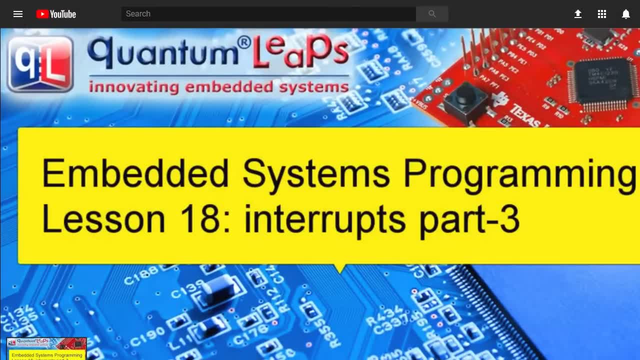 from the previous lesson so that you can have multiple background loops running seemingly simultaneously. To follow along today's lesson, I highly recommend that you watch again lesson 18 about interrupts so that you have it fresh in your memory. In terms of the software, you need the previous lesson. 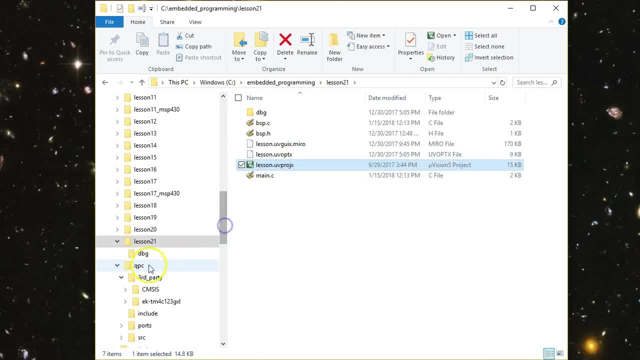 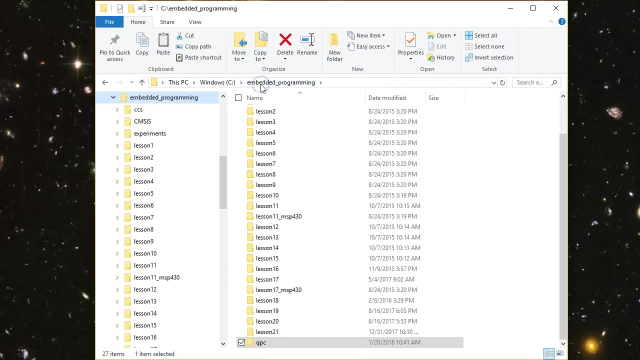 The previous lesson 21 explains how to download and install all this software, including the Arm-Kyle-Microvision development toolchain. With these prerequisites in place, make a copy of the lesson 21 directory and rename it to lesson 22.. 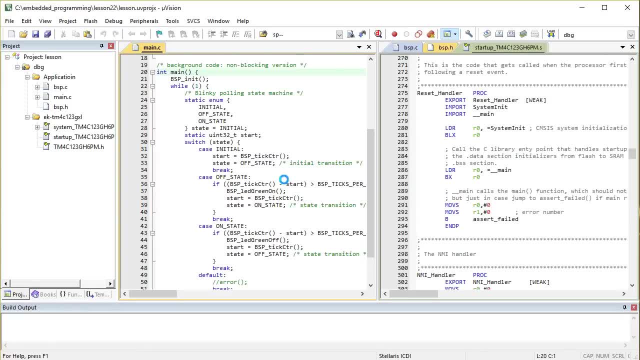 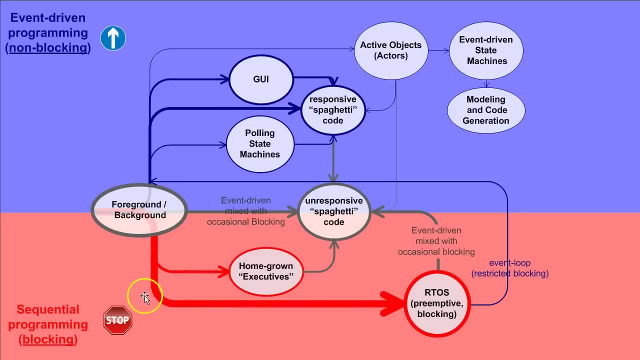 Get inside the new lesson 22 directory and double-click on the Microvision project lesson to open it. To remind you quickly what happened so far: in the last lesson you've learned the basic foreground-background architecture and you saw that it can be implemented with sequential 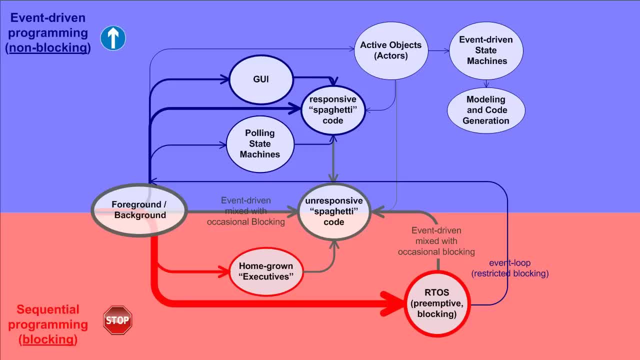 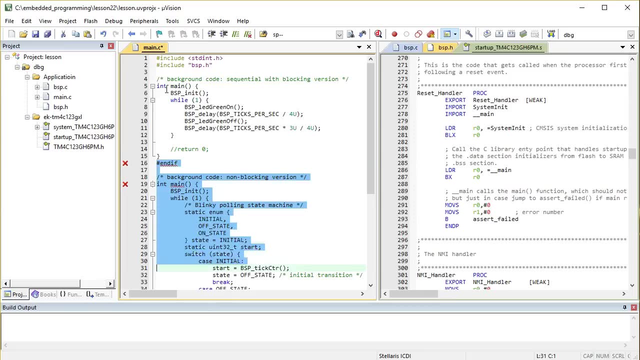 blocking code and with event-driven non-blocking code. For this lesson, you revert to the sequential code and delete the event-driven alternatives. For this and the couple of next lessons, you are going to focus on the sequential architectures, such as the RTOS. I promise to go back to the event-driven architectures in the future. 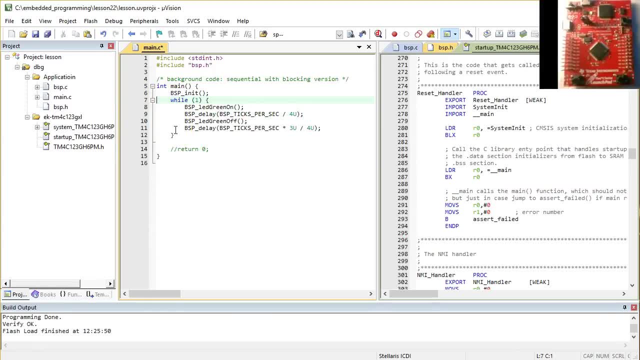 lessons. The sequential code from last time simply blinks the green LED on your Launchpad board. Today's challenge is to extend this basic architecture to also blink the blue LED available on your board, but to do it independently and simultaneously with blinking the green. 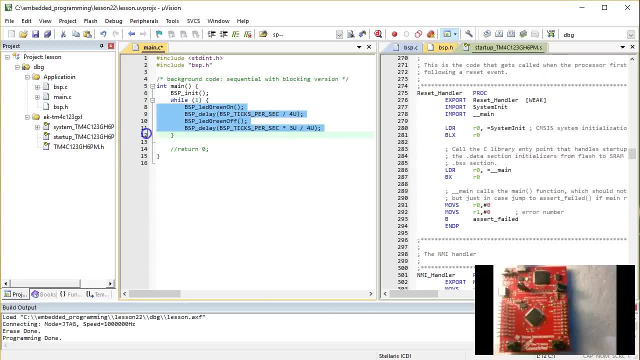 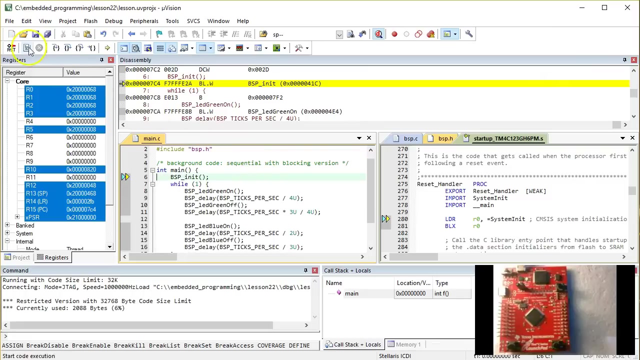 LED. The first naive attempt could be to just copy and paste the code for the green LED and replace the LED color and perhaps also change the on and off delays. When you compile and load this code to the board, you find out that it blinks both LEDs, but not simultaneously. 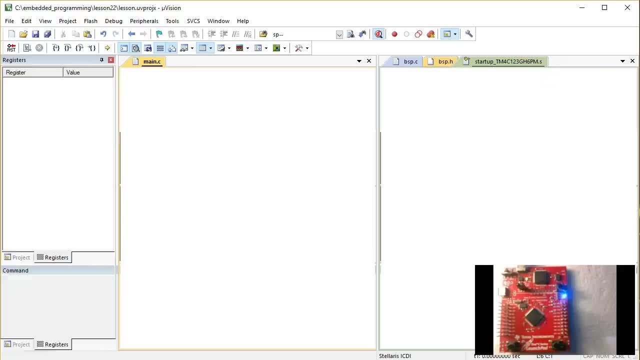 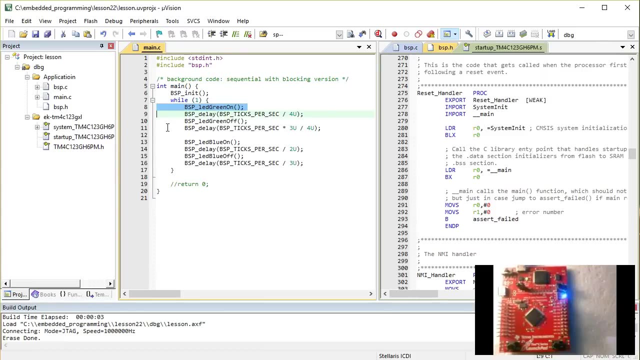 Instead, the LEDs are turned on and off in sequence: first the green LED and then the blue LED. Of course, this is exactly the nature of the sequential code you created. All you did just now was to extend the hard-coded sequence of events to include also switching the blue LED on. 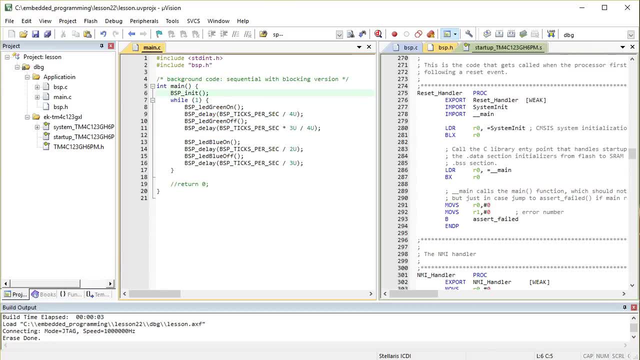 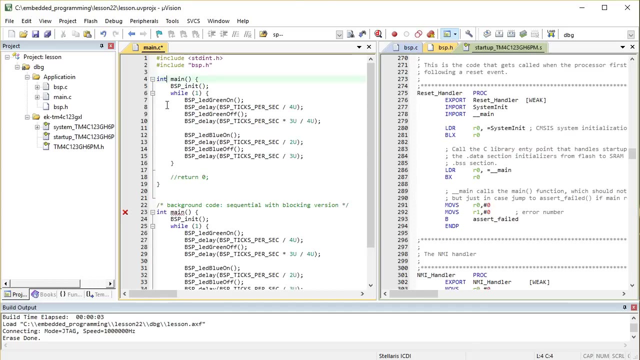 and off To blink the LEDs truly independently, while preserving the simple sequential structure of the code. you would need not one but two background loops running somehow simultaneously. To explore this possibility, let's create two main functions called mainblinky1 and. 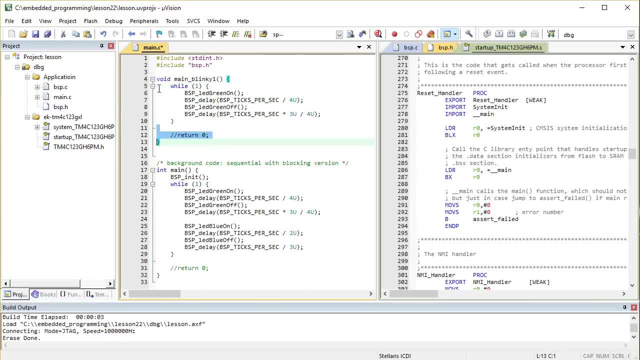 mainblinky2.. Each of these functions having the usual structure of the while-1 endless background loop. Now, in the original main program, you need to call these functions so that the compiler won't eliminate the two main functions as unused code. 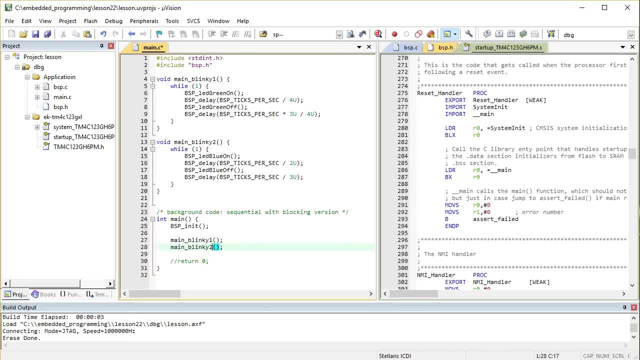 However, it turns out that you cannot simply call the functions one after another, because the compiler is so smart that it will still eliminate the second call as unreachable. So let's try this. Here we go: The first call will not return, because it knows that the first call never returns. 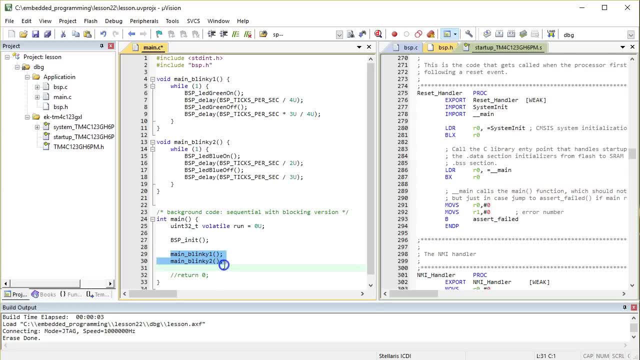 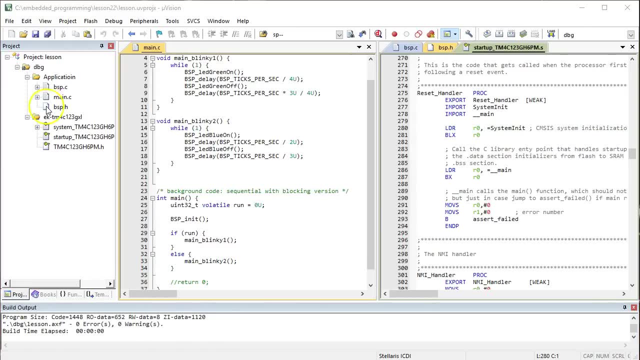 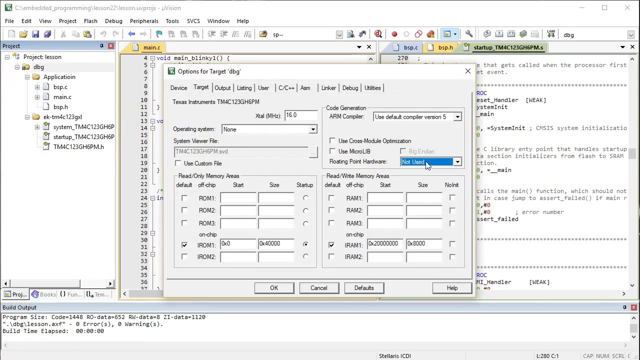 To prevent this, you can add an if-statement controlled by a volatile variable like this: Before you run this code, however, please open the Project Options dialog box and turn off the use of the floating-point hardware, similarly as you did in lesson 18.. 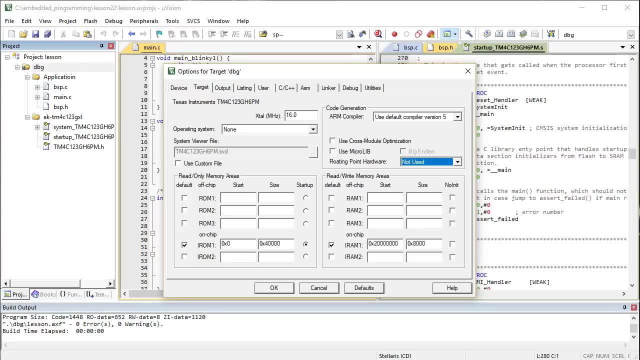 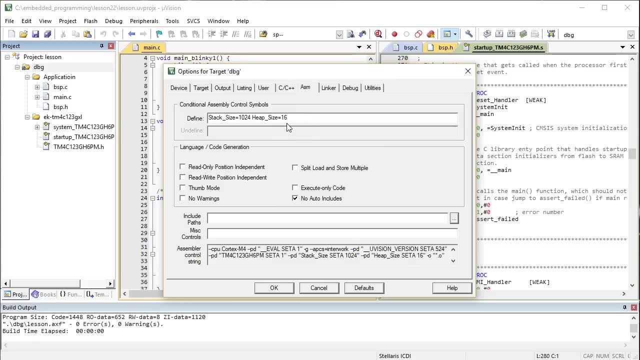 This is to simplify the way CPU handles interrupts, which will turn out to be important for the following discussion. Also, as you can see, the first call never returns. Also, as you are at it, please make sure that you have a non-zero heap size. 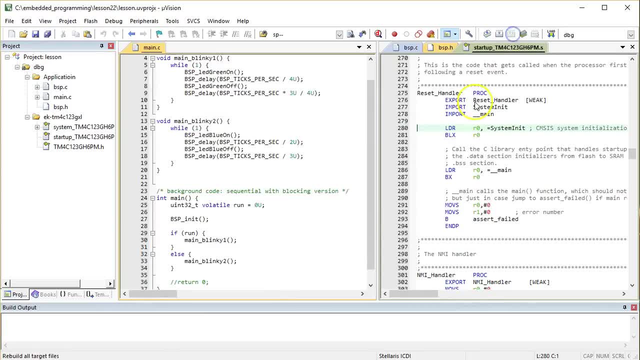 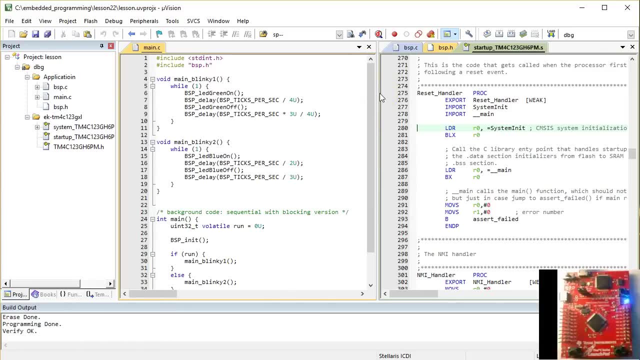 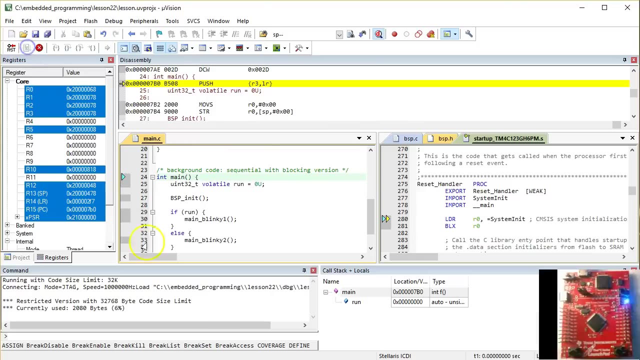 Again, it turns out that the Kyle debugger likes to have some heap space for the so-called semi-hosting feature. With these changes, let's open the code in the debugger. When you run the code free, you can see that it only blinks the blue LED from the main. 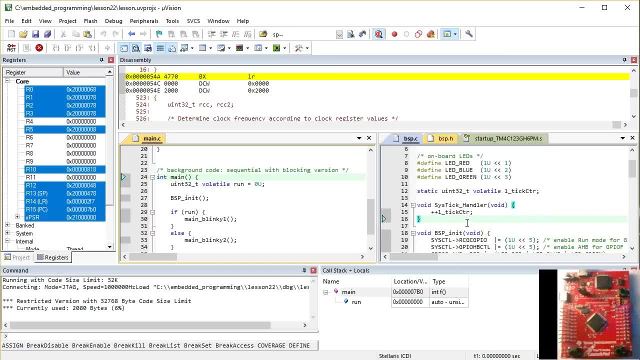 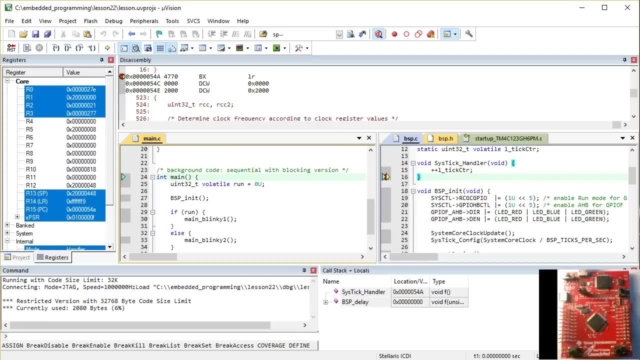 Blinky2 function, But let's place a breakpoint at the end of the SysTick interrupt handler in BSP. Let's run the code again. Let's run the code again. As you remember from the previous lesson, you have configured this interrupt to fire. 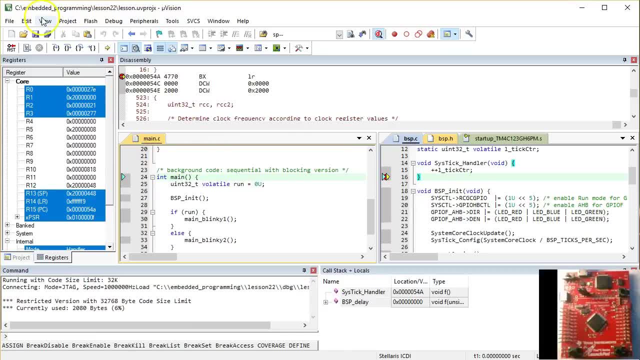 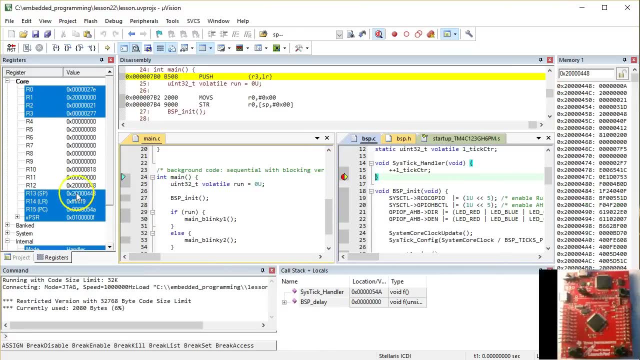 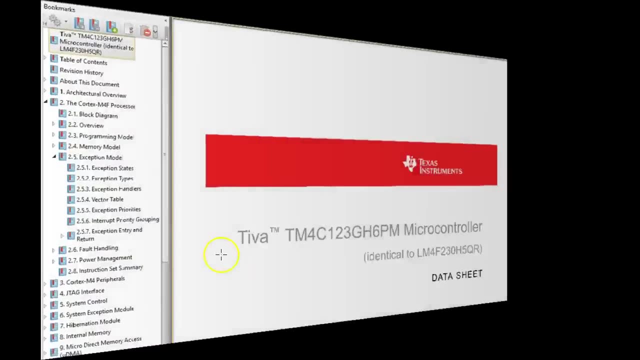 a hundred times per second. When you hit the breakpoint, open the Memory 1 view and dock it along the right side of your screen. Scroll the memory to the address of the Stack Pointer Register. Now, in lesson 18 about interrupts, you learned about the very specific stack frame generated. 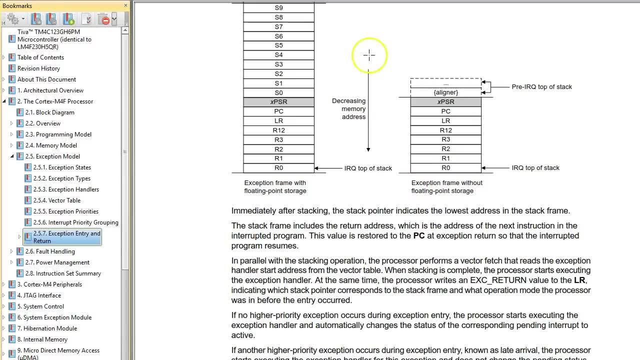 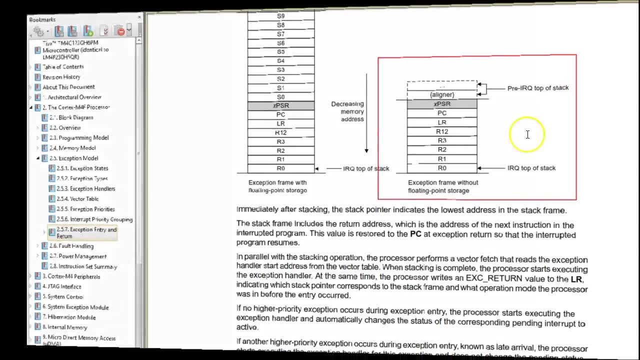 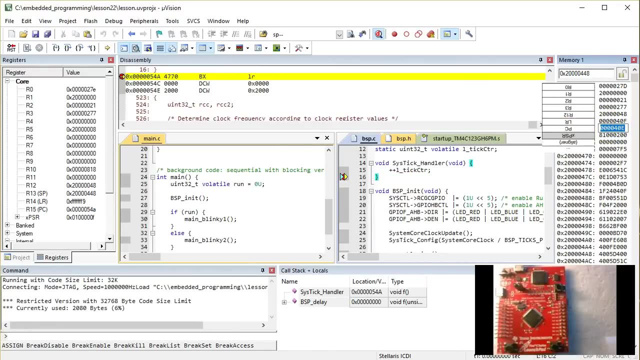 by the ARM Cortex-M exceptions such as interrupts. To quickly refresh your memory, I will grab the layout of the interrupt stack frame from the TIVA-C datasheet. I will then align the interrupt stack frame with your stack memory view, remembering to 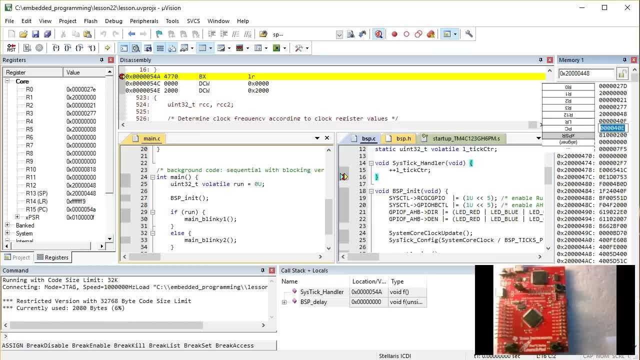 flip it upside down because the ARM stack grows toward the lower memory addresses. As you can see, the seventh stack entry from the top contains the program counter PC. This value will be loaded to the PC register upon the return from the memory register. 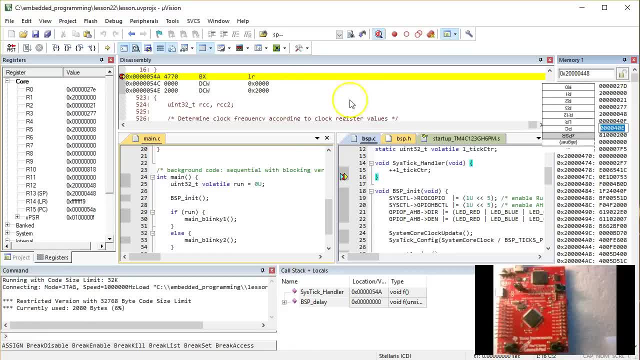 This value will be loaded to the PC register upon the return from the memory register. This value will be loaded to the PC register upon the return from the memory register. This value will be loaded to the PC register upon the return from the interrupt. This value will be loaded to the PC register upon the return from the memory register. 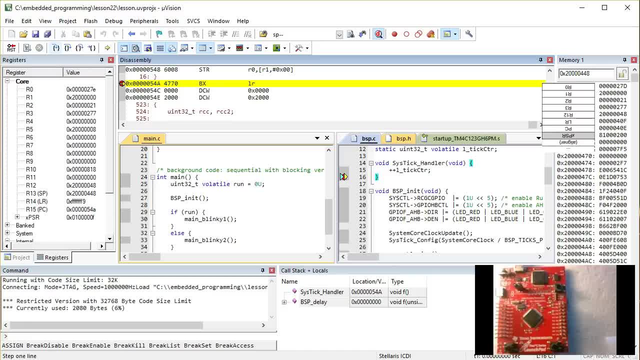 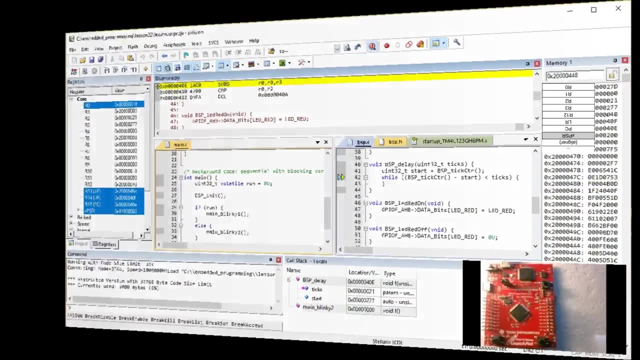 So, for example, here the PC will be loaded with HEX40E, which you can easily test experimentally by simply stepping through the BXLR instruction and watching where the interrupt returns to, And indeed it does return to- the address HEX40E. 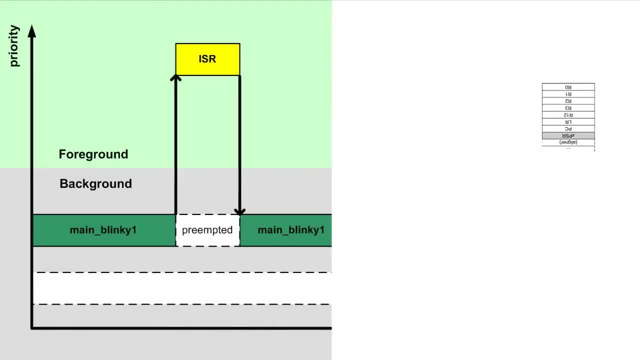 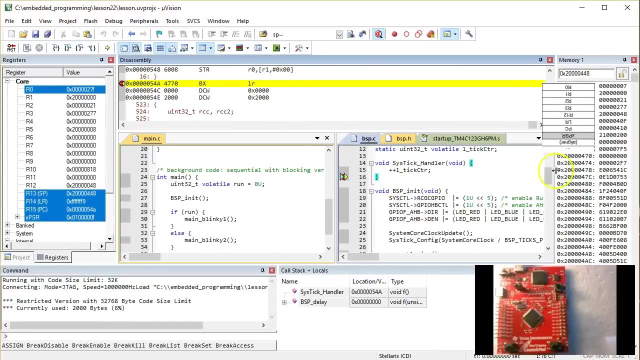 This is a regular interrupt. return to exactly the point of preemption. But now, when your breakpoint in SysTick Handler is hit again, Let's cheat and change the stack entry corresponding to the PC to the address of your main blinky1. 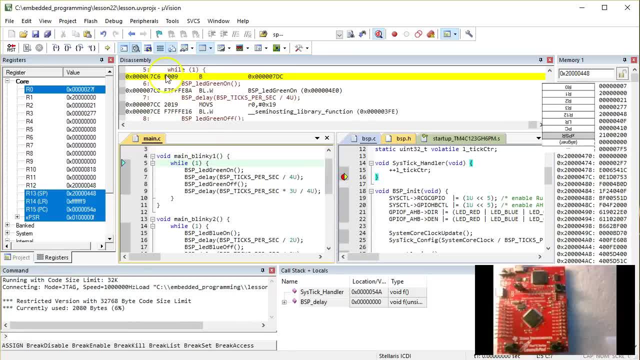 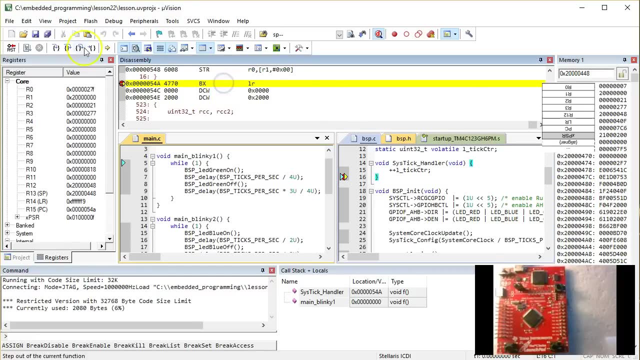 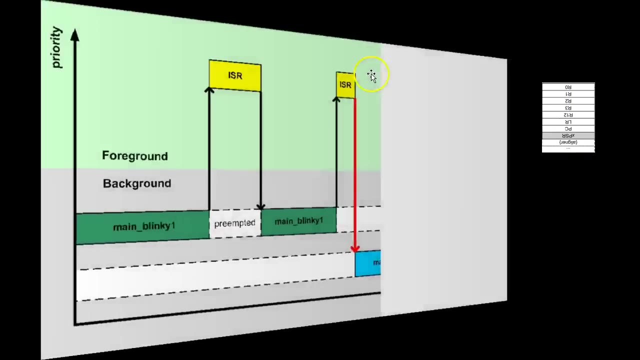 function, which happens to be 7c6.. When you execute the return from interrupt instruction BXLR, this time you can see that you indeed returned to main blinky1.. This means that you are returning to a different point than the original point of preemption. 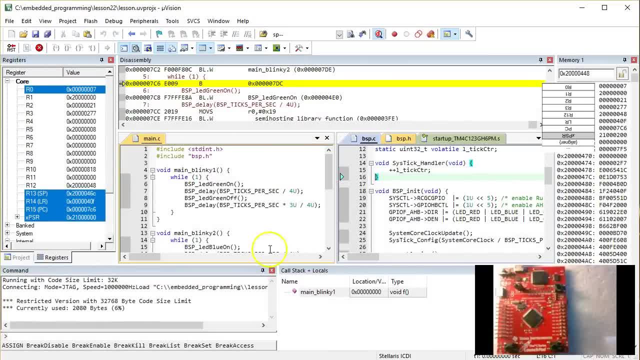 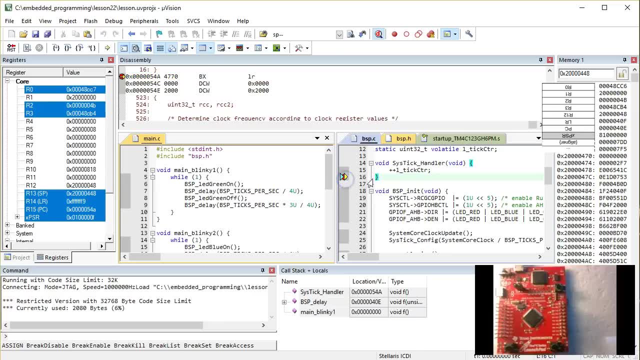 When you remove the breakpoint in SysTick Interrupt and let the code run free, you can see that you are now blinking the green LED. Of course you can repeat the process again, but this time go back to executing main blinky2.. And indeed, you now blink the blue LED. 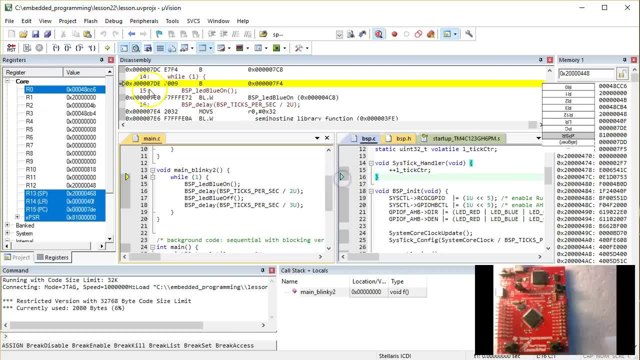 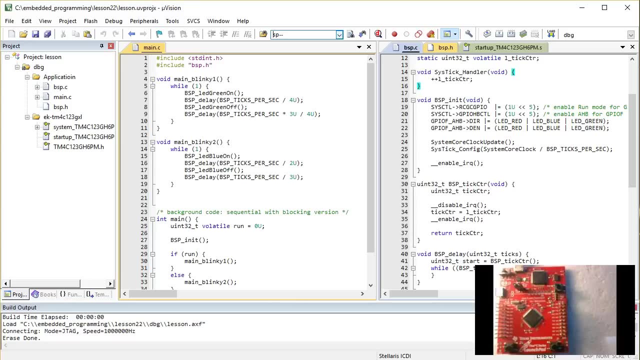 Here. I need to warn you, however, that what you've just done is not quite legal and will not really work with a more complex code, as I will explain in a minute. So let's go back to SysTick. And indeed, you now blink the blue LED. 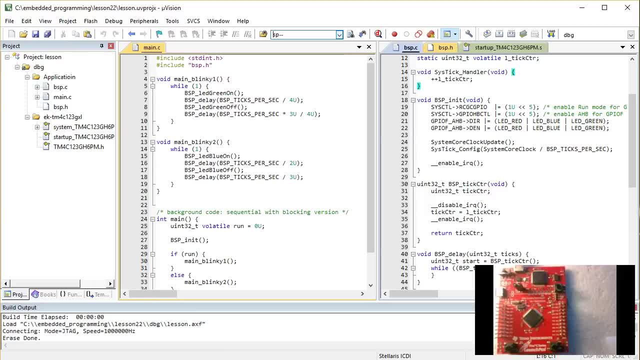 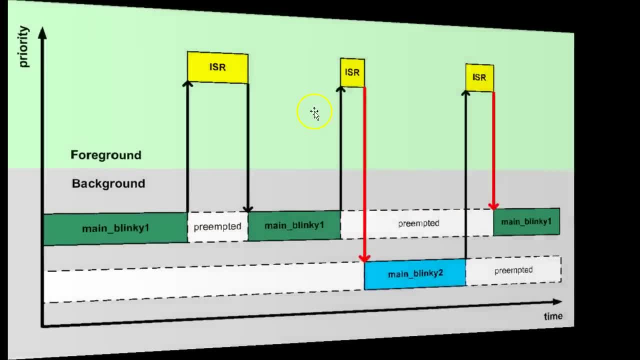 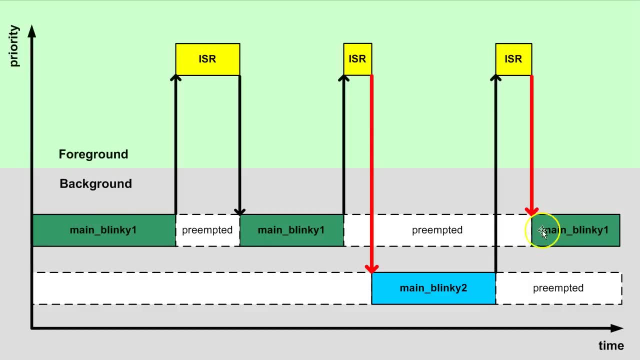 But already at this point the exercise allows you to make a couple of interesting observations. First of all, you can see that such switching the CPU between executing multiple background loops should be possible. Second, the exercise points you to the general mechanism for such CPU context switching. 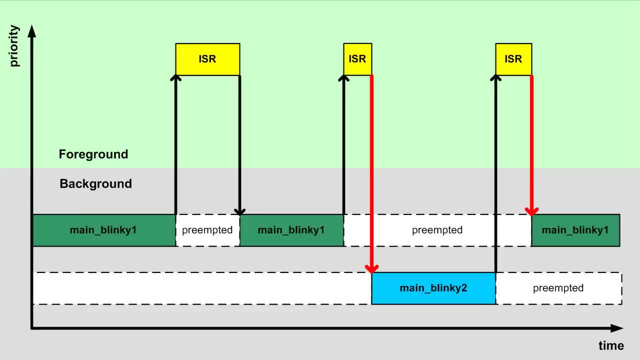 which is to exploit the interrupt processing hardware already available in your processor. And third, the general idea of multitasking on a single CPU, which is to switch the CPU between executing different background loops, like your main blinky 1 and main blinky 2, here. 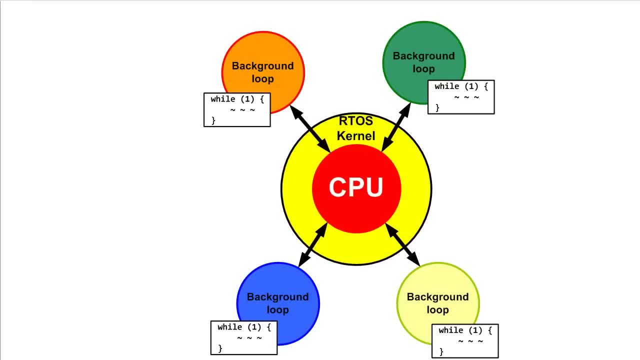 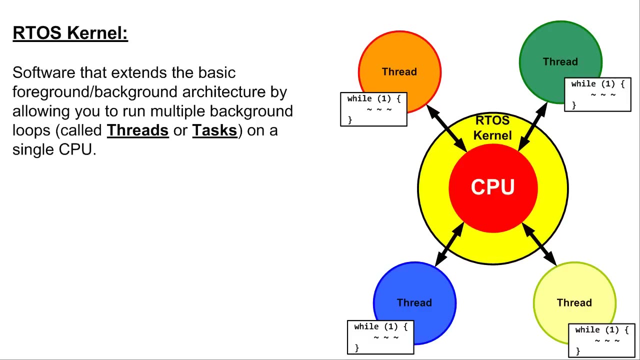 So far in this lesson you've been doing the switching manually, but the process can be automated in special software called the Real-Time Operating System Kernel, or RTOS Kernel for short. A simple definition of an RTOS Kernel is that it is software that extends the basic foreground-background. 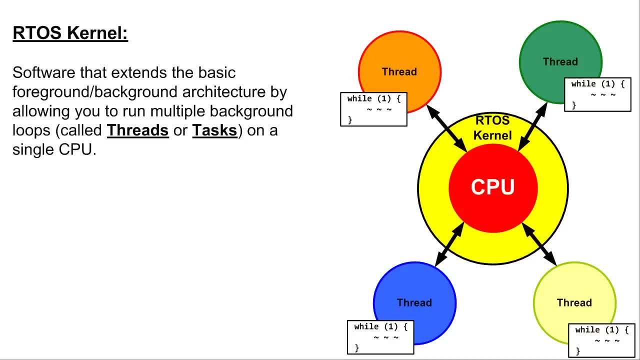 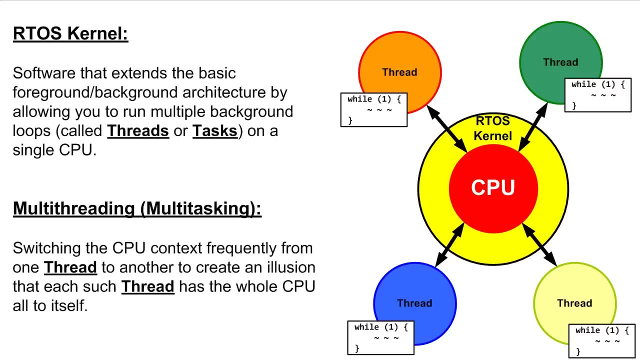 architecture by allowing you to run multiple background loops, called threads or tasks, on a single CPU. Another term that you should learn is multithreading or multitasking, which is switching the CPU context frequently from one thread to another to create an illusion that each such thread 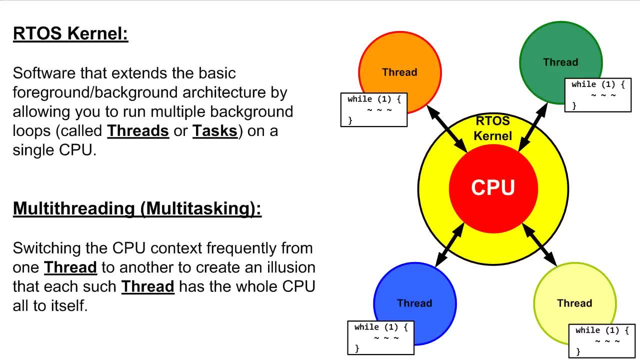 has the whole CPU all to itself. Both these definitions use the term thread, but I want you to remember that these threads are essentially the background loops from the foreground-background architecture. Now, in the remaining part of this lesson, let me go back and explain why changing the 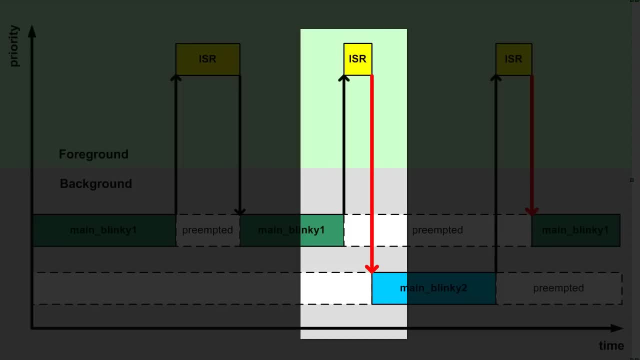 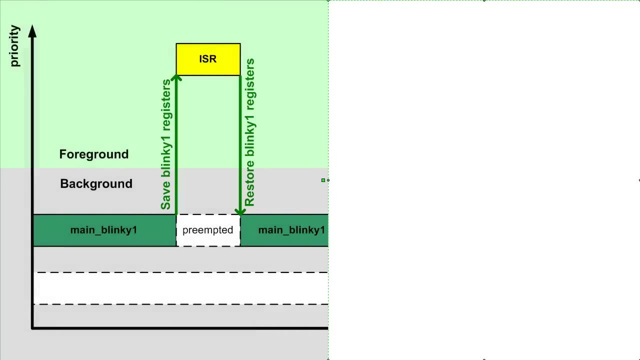 PC register value on the stack was illegal and what you really need to do to switch context cleanly from one thread to another. To illustrate the problem, let me use colors for the registers that are saved and restored by an interrupt. Here, for example, I use green for the registers that are saved and restored by an interrupt. 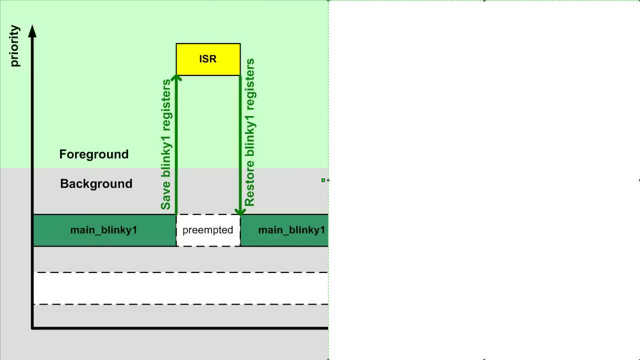 Here, for example, I use green for the registers that are saved and restored by an interrupt, the registers of blinky1, because it blinks the green LED. As you can see, in the case of the regular interrupt preemption, you save registers for. 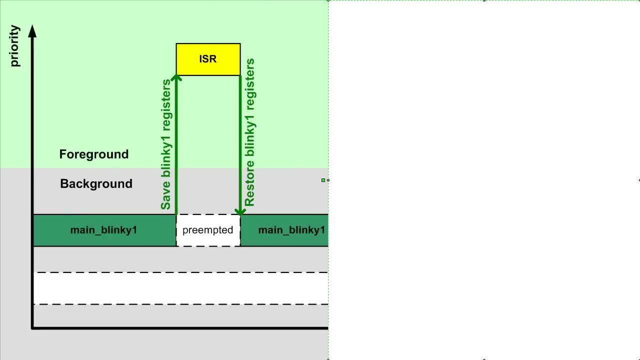 the blinky1 thread and restore the registers for the same blinky1 thread. As long as you actually return to the blinky1 thread, everything is OK. However, when you manually modify the return address, you are returning to the blinky2. 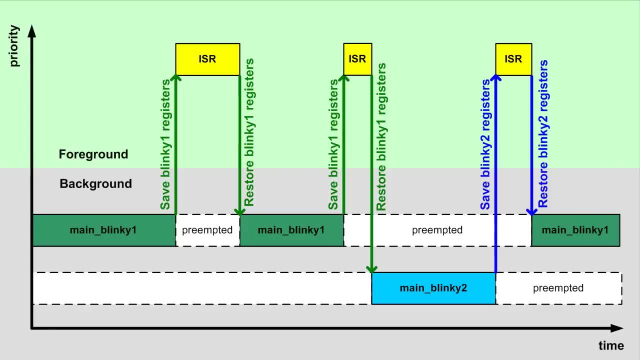 thread, but you still restore the registers saved originally for the blinky1 thread, which is exactly the illegal part. It happens to just work for the dead simple blinky threads, but it can and will break down for more complex threads that use more registers. 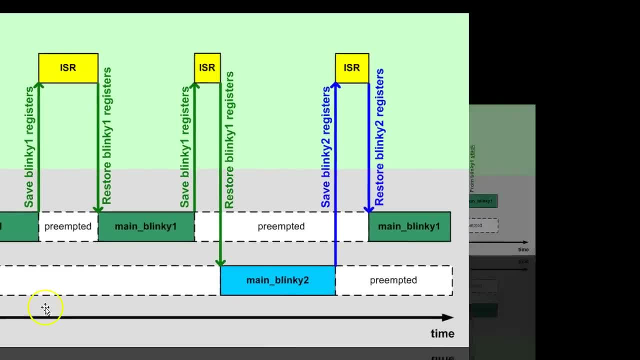 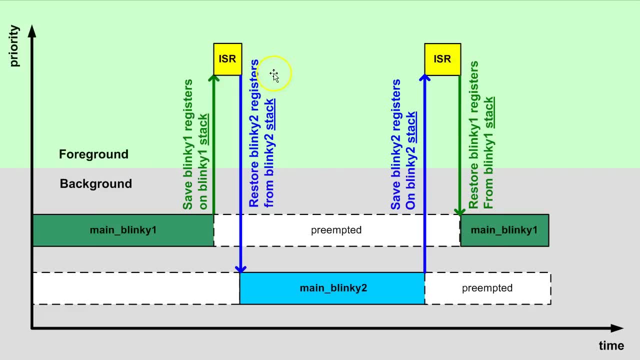 So now you might have a better idea how to fix it. Well, you need to keep the register sets for different threads separate. In other words, the registers saved for blinky1 cannot be restored for blinky2, and vice versa. What that means is that you need to use a separate. 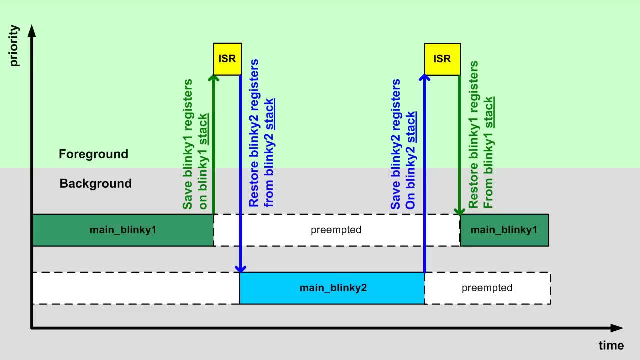 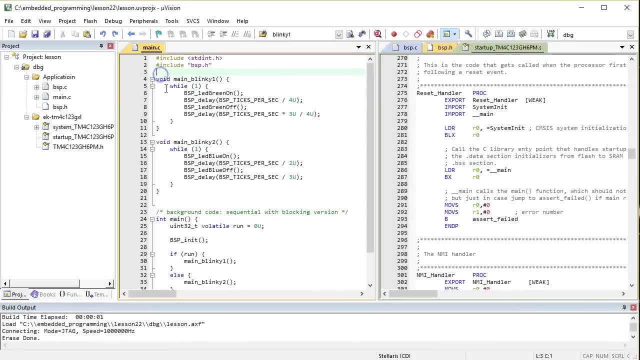 private stack for each thread. Again, it might sound complicated at first, but really isn't. as you will see in the following experiment, You can quite easily add a stack to a thread, because it is really nothing more than an area in RAM and a pointer that points to the current top of that stack. 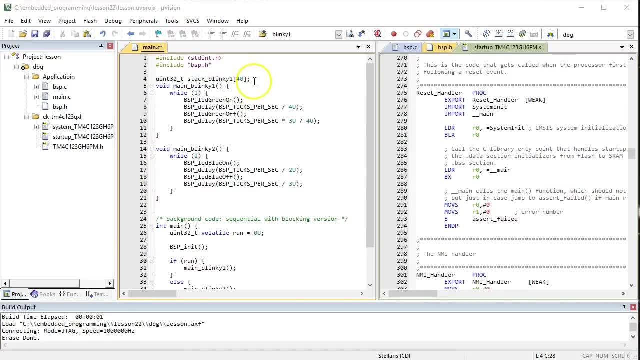 In C, such a memory area can be represented as an array of Uint32-bit words, corresponding to the 32-bit registers of the CPU, plus a stack pointer. Let's initialize the stack. This is the stack pointer to point one word beyond the end of the stack array, because 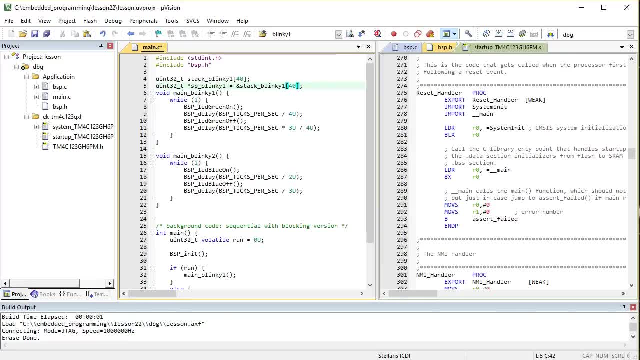 on the ARM CPU the stack grows down. That is from the end of your stack array to its beginning. You need to provide a similar stack for the blinky2 thread as well. Now in the main program, you no longer need to call the thread functions. 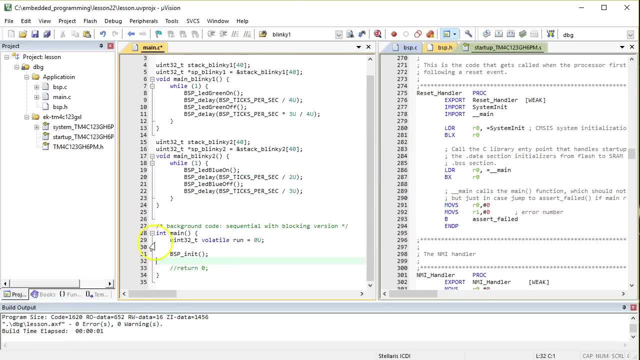 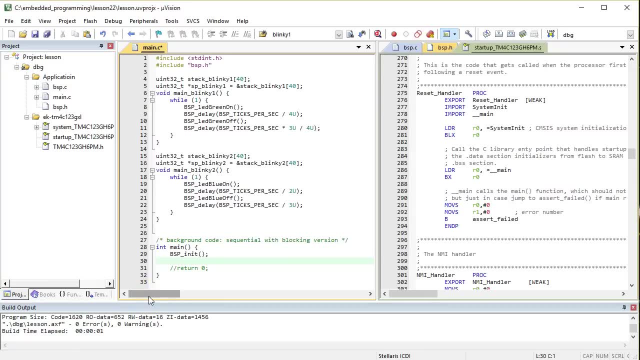 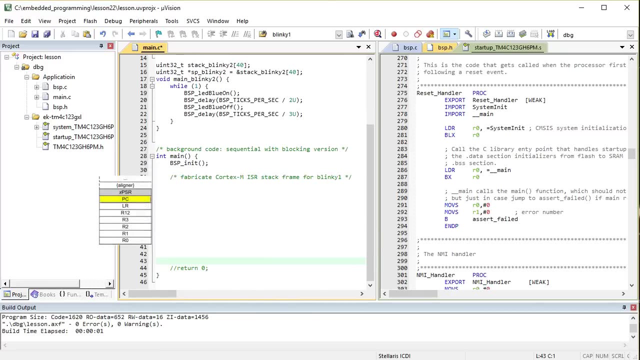 Instead, you need to prefill each thread's stack with a fabricated Cortex-M interrupt stack frame. The goal is to make the stack look as if it was preempted by an interrupt just before calling the thread function. Therefore, you can use again the ARM exception frame layout from the datasheet as your template. 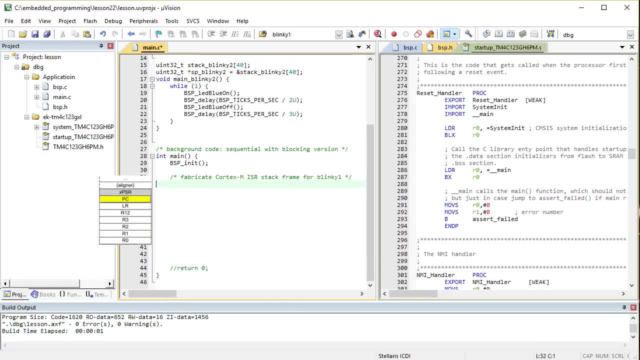 You start from the high memory end of the stack, because the ARM stack grows from high to low memory. Also, the ARM CPU requires that the ISR stack frame be preempted by an interrupt just before calling the thread function. This is the case here because the stack array was sized at 40 32-bit words, which 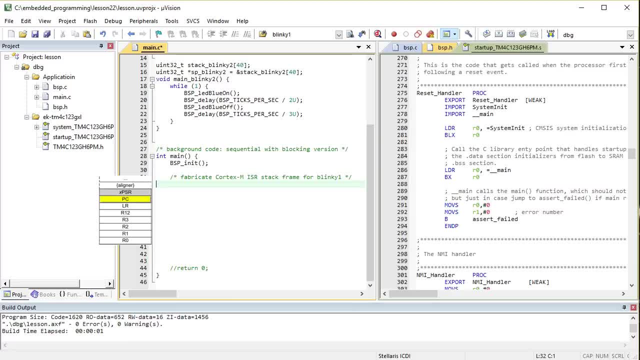 aligns at the 8 of 8-byte boundary. This means that the aligner stack entry is not necessary. Finally, the ARM CPU uses the full stack, which means that the stack pointer points to the last used stack entry, as opposed to the first free entry. 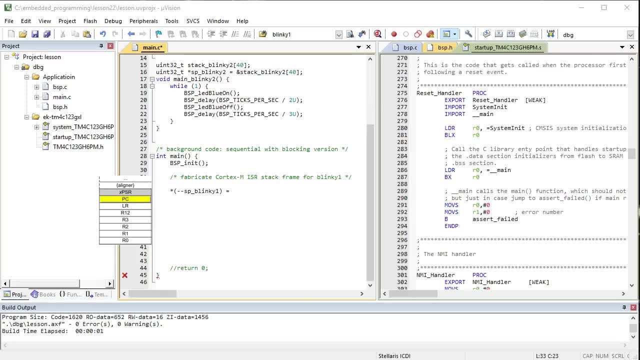 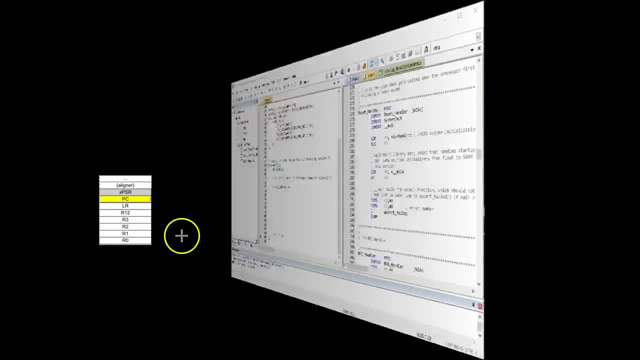 Therefore, to add a new stack entry, you first decrement the stack pointer to get to the first free location And then you dereference it to write a value to this location. The first value you write is the fabricated program status register in which you need: 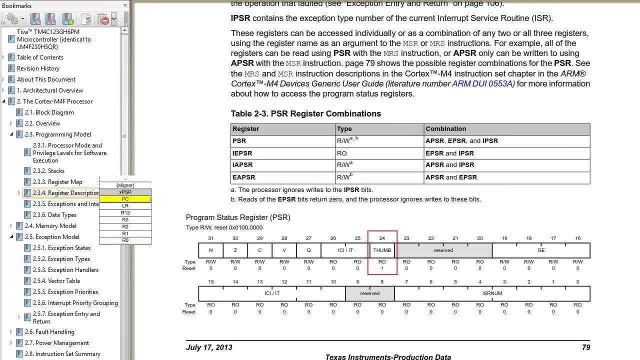 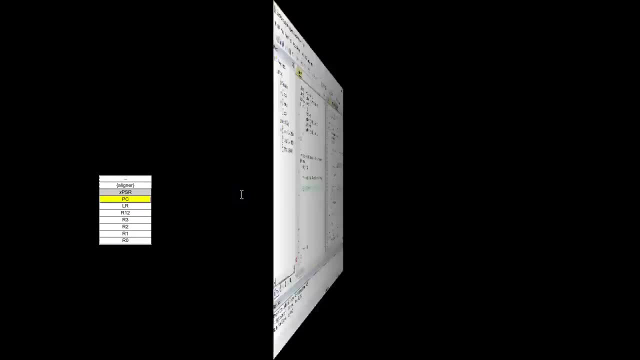 to set just one bit, number 24.. This bit corresponds to the thumb state of the processor. The Cortex-M processor cannot be really in any other state, such as the ARM state, but for historic reasons the XPSR register must have the thumb bit set. 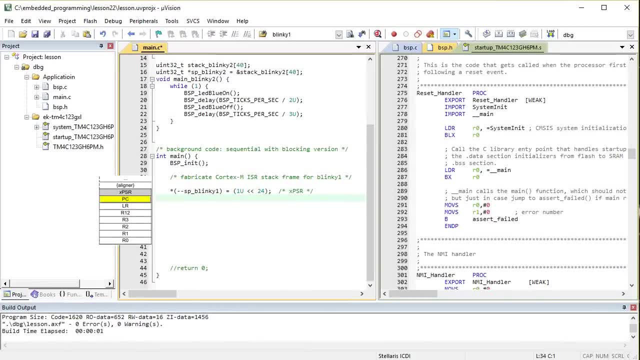 The next value on the stack is the PC. This is the return address from the interrupt and, as you saw from your earlier experiments, it needs to be set to the address of the Thread function. I have not explained yet in this course that the C language allows you to take an address. 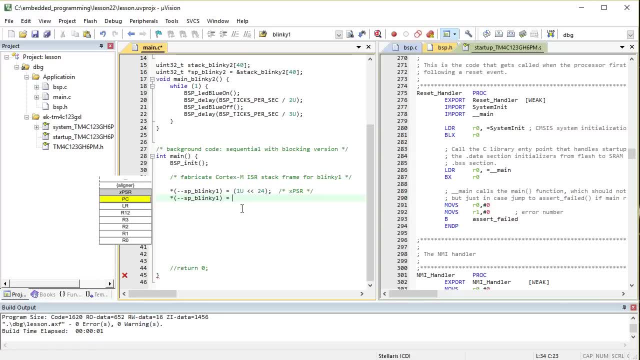 of a function using exactly the same ampersand operator as taking an address of a variable. The address of operator applied to a function produces a pointer to function, which I will explain in more detail in a future lesson about state machines. For now, you need only to write the address of the Thread function. 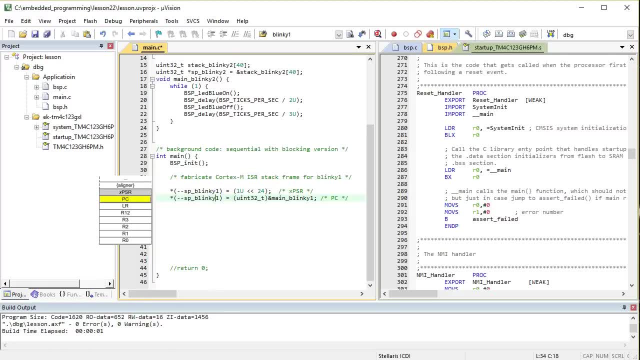 Only to understand that such a pointer can be created but must be cast on uint32 to fit on your stack. The other registers in the ISR stack frame do not really matter for the proper calling of the Thread function, because a thread does not return. 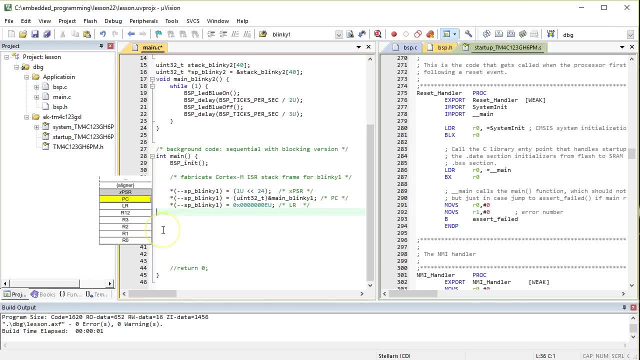 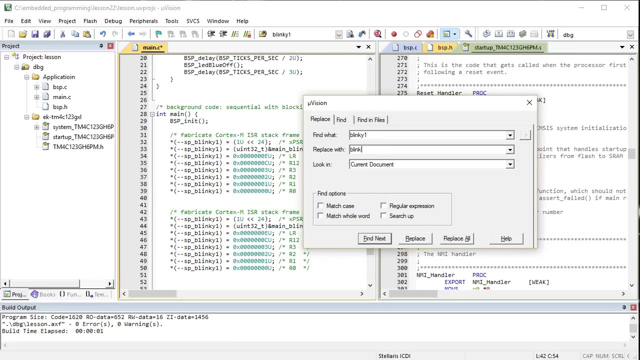 But for testing purposes you can initialize the stack with numbers corresponding to the register number. This will help you to easily recognize the stack frame in the debugger. You initialize the stack for the blinky2 thread in exactly the same way, Except you use the address of the blinky2 thread function for the PC register value. 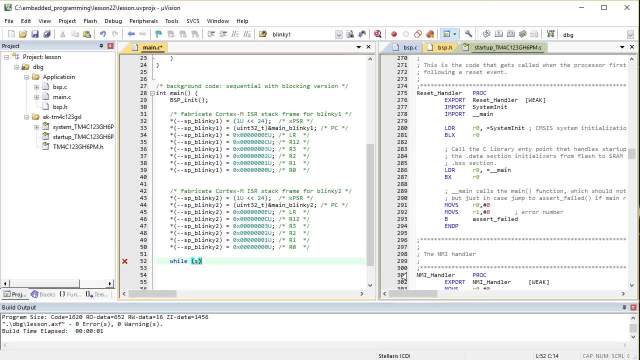 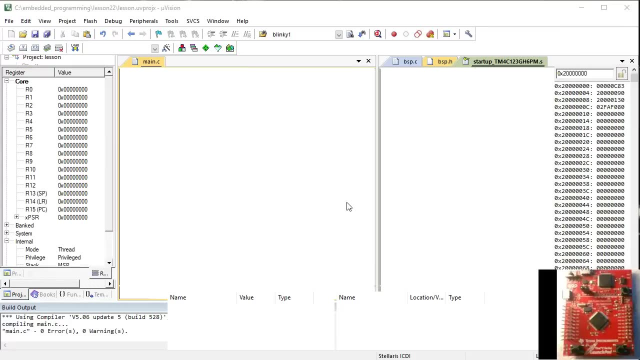 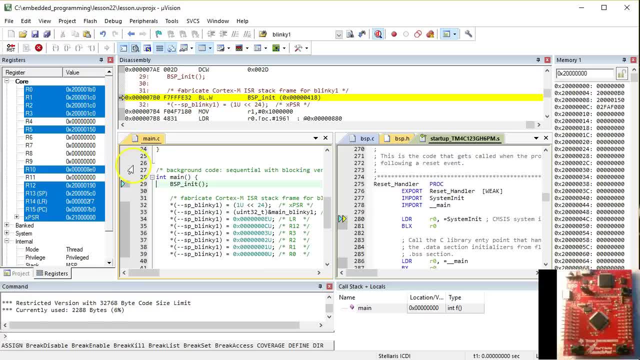 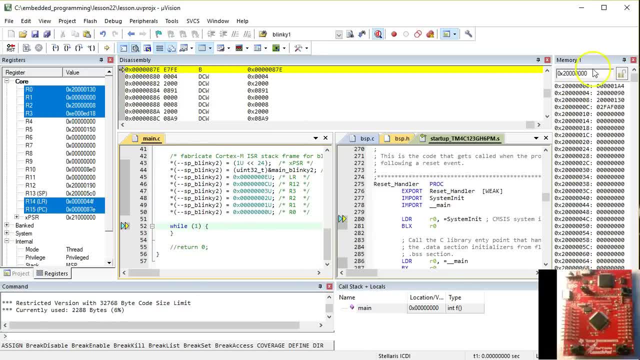 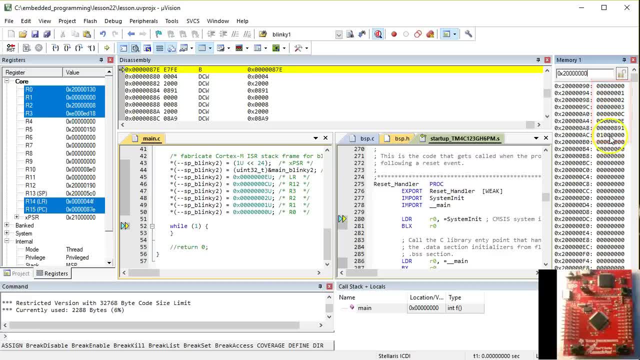 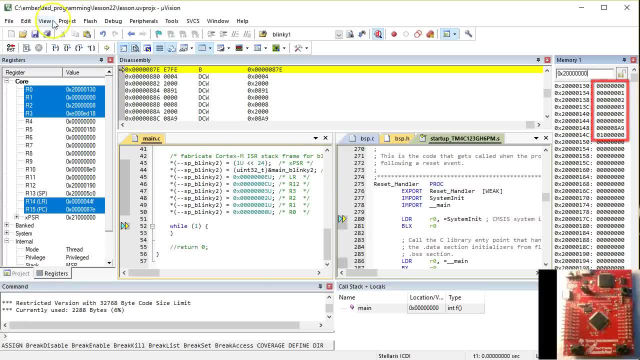 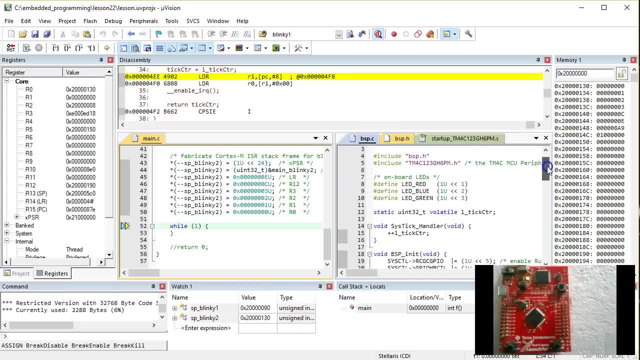 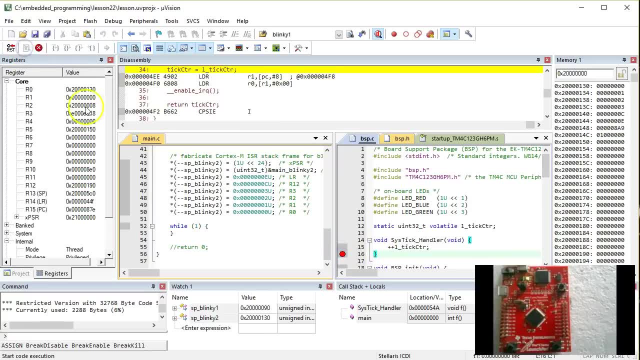 Now comes the most interesting part, and I can only imagine that you must be hanging by the edge of your seat for what's about to happen. Set your usual breakpoint at the end of SysTick and when it is hit. 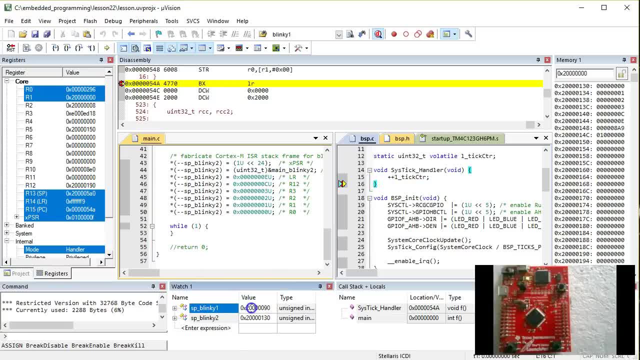 you switch the CPU stack from the original main C stack to one of the private Blinky stacks, say Blinky 1.. To do this, you simply manually change the SP CPU register to the value of the SP Blinky 1 variable. 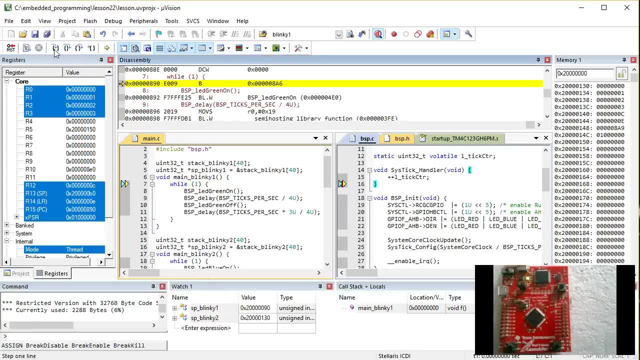 Now, when you step through the BXLR returned from interrupt instruction, you can see that you end up in the Blinky 1 thread and when you remove the breakpoint from SysTick you blink the green LED To change the context to the Blinky 2 thread. 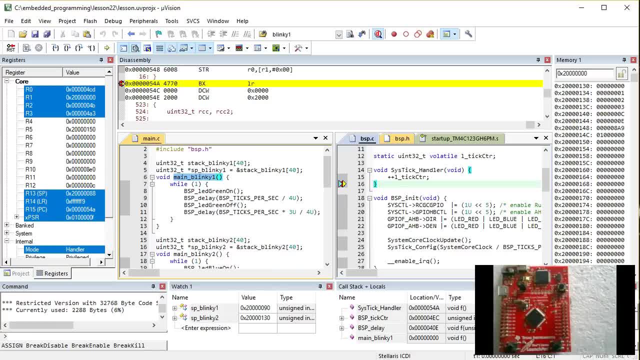 set the breakpoint at the end of SysTick again, and this time you will switch the stack to Blinky 2.. But before changing the SP register in the CPU, copy the current value of the SP from the CPU into the SP Blinky 1 stack pointer variable. 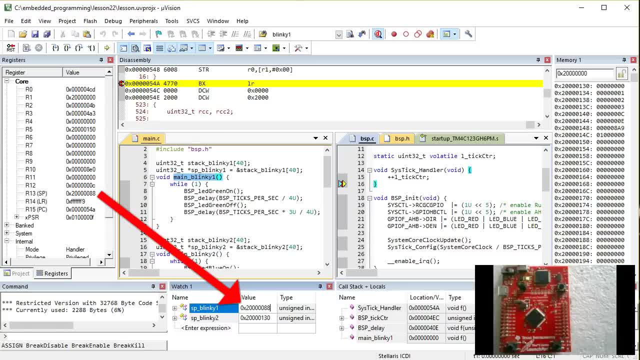 because this really is the current top-off stack for the Blinky 1 thread, and so you need to update the stack pointer before switching away from this thread. Only now you can overwrite the SP register with the top-off stack of the next Blinky 2 thread to execute. 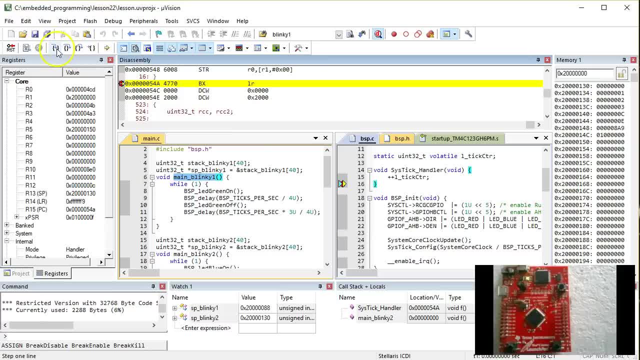 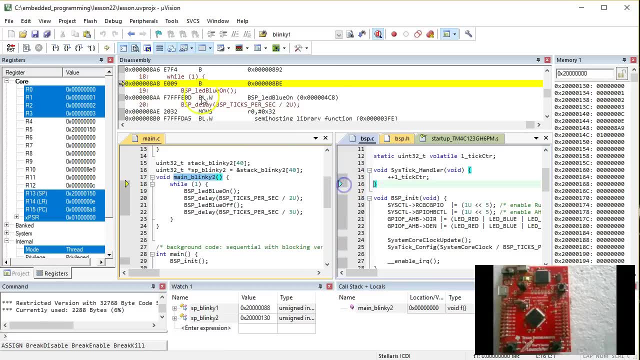 When you step through the BXLR instruction, you can see that. now you return to the Blinky 2 thread. When you remove the breakpoint and run the code again, you can see that the blue LED starts blinking. so you are indeed running the Blinky 2 thread. 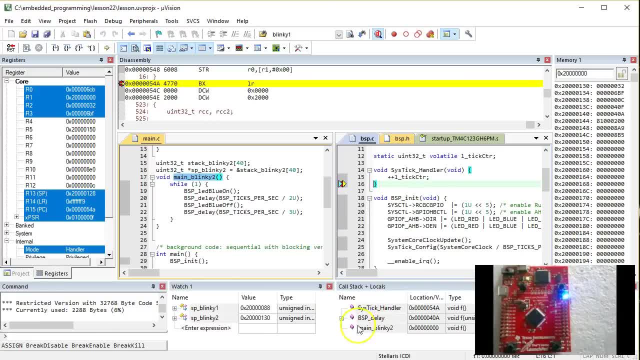 So now I hope you are getting the hang of it. Your manual procedure of switching the CPU context is to break at the end of the SysTick interrupt. copy the current value from the SP register into the stack pointer variable. 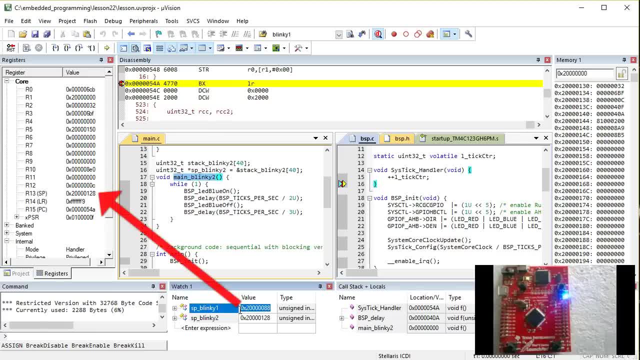 corresponding to the currently executing thread and to copy the other thread's stack pointer to the SP register. Please note, however, that you no longer need to mess with the stack content in memory. Please also note. 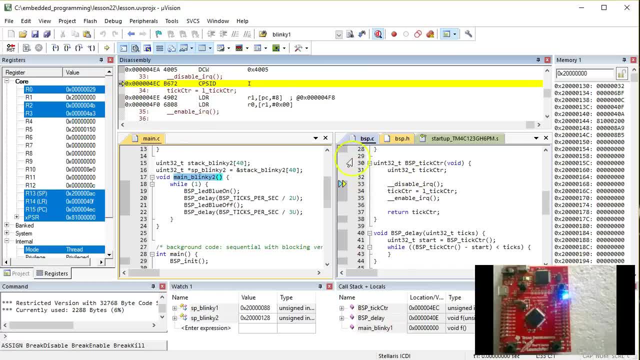 that if you switch to the Blinky 1 thread now, you resume it at precisely the point of preemption by the SysTick interrupt and not at the beginning of its thread function. For example, here you return to a specific location. 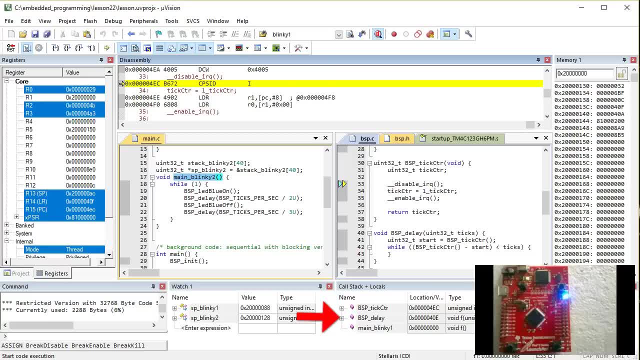 in the BSP tick counter function, which was called from a specific location. in the BSP delay function, which was called from main Blinky 1 thread. All this information is preserved on the private Blinky 1 stack When you run the code free. 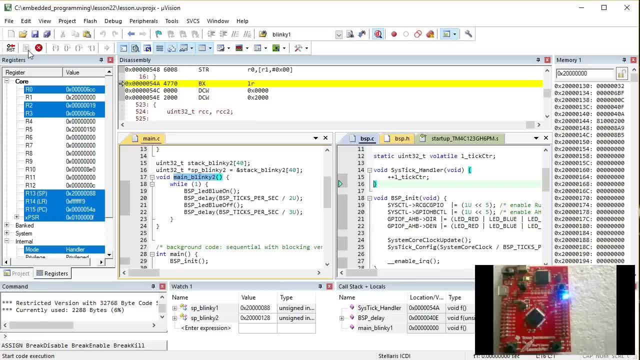 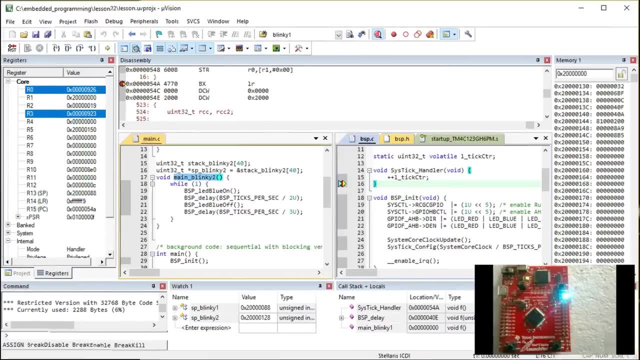 the two threads execute now independently. For example, here the Blinky 1 thread runs while Blinky 2 is preempted with the blue LED turned on. The timing diagram illustrates the new way of context switching, using a separate private stack for each thread. 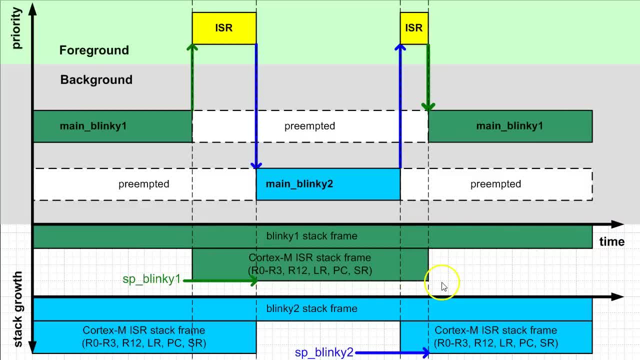 As you can see, you no longer mix registers. Instead, the registers for Blinky 1 thread are stored on Blinky 1 stack and subsequently restored from the same Blinky 1 stack. The same goes for Blinky 2.. 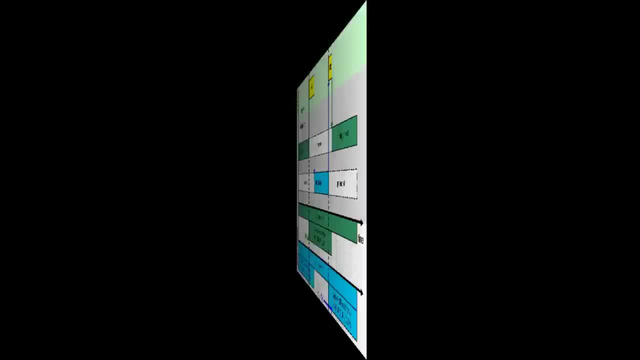 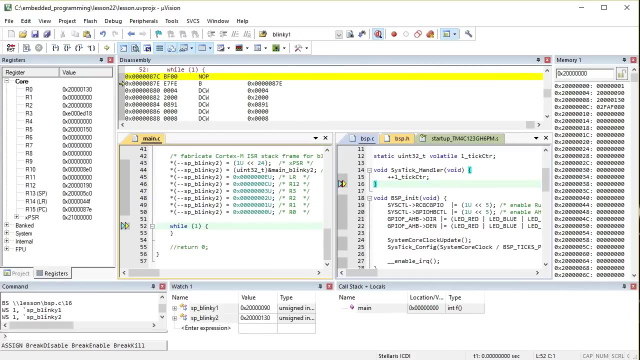 or any other thread that you might add to the system. All of this looks very promising as the way to implement the context switch, but you are not quite out of the woods yet. The remaining problem is that your context switch can still clobber some CPU registers. 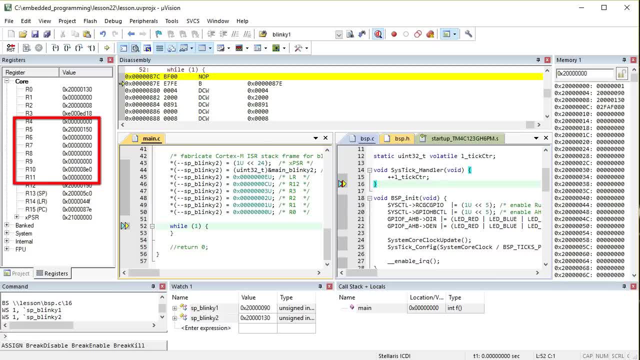 so the CPU state is not quite correctly restored. before resuming a given thread. To understand why, recall from lesson 18.. that the Cortex-M exception stack frame corresponds to the ARM application procedure, call standard AAPCS. 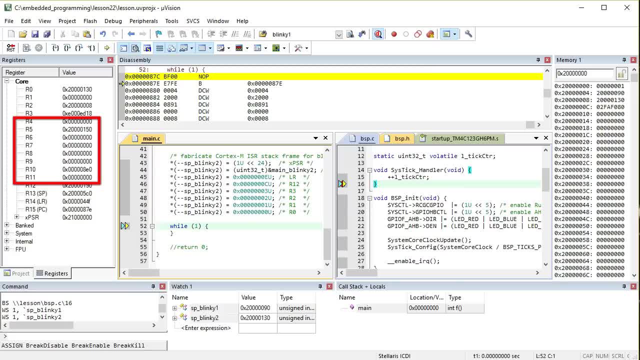 in that it stores only the registers that are allowed to be clobbered by a function call, but does not store registers R4 through R11. which must be preserved by a function call. This works for interrupt service routines- ISRs. 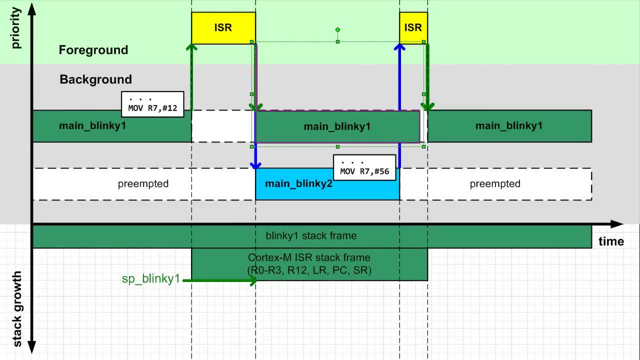 because an ISR must necessarily run to completion before returning to the preempted code. For example, suppose that Blinky 1 thread code uses the R7 register which, as you can see, is not saved in the Cortex-M ISR stack frame. 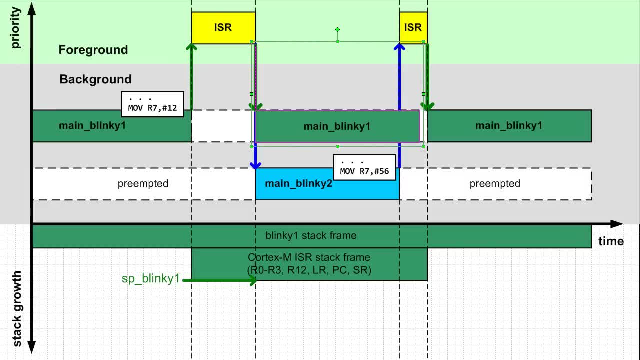 The ISR might be also using R7. but it must save it and restore before returning. This works just fine, but only when the ISR is the only code executed while a thread is preempted. But in your case, the ISR does not return to the preempted code. 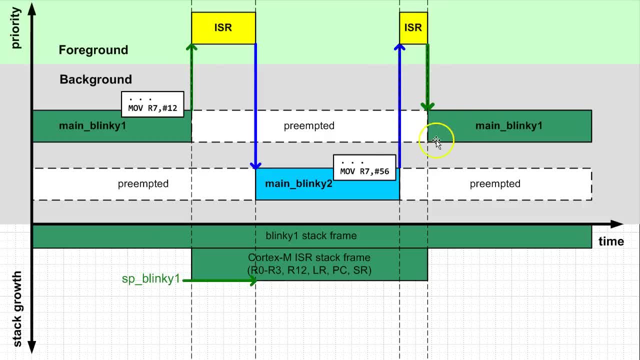 but rather to another thread, Blinky 2.. This other thread can also use the R7 register and, as any function is also obligated by the AAPCS to restore the R7 upon its return. But you are not executing the whole thread function. 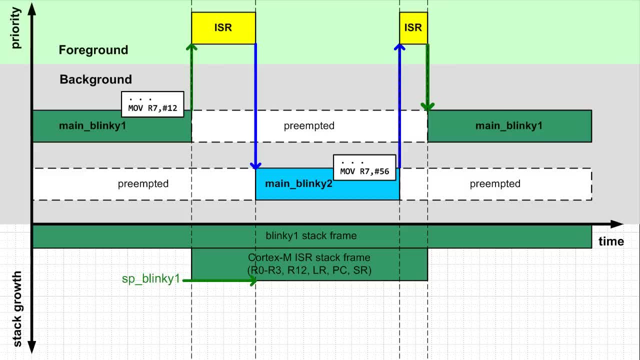 but rather just a piece of it. This piece of code doesn't need to comply with the AAPCS and it can change the value in R7.. The result is that by the time Blinky 1 resumes execution, the R7 register might be clobbered. 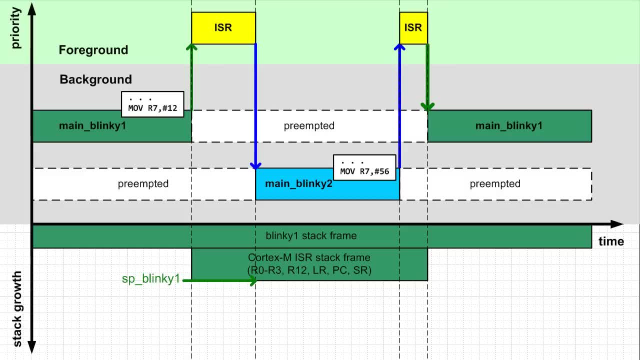 which is a problem. Of course, the same argument can be made about any of the registers R4 through R11.. The solution is to save the remaining eight registers, R4 through R11, on the thread stack at the end of the ISR. 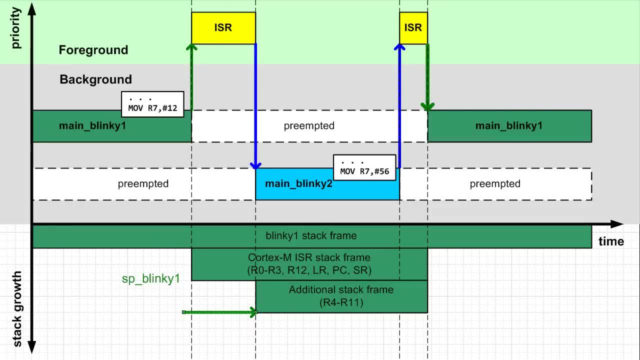 right before switching the context away from the thread. These registers must then be restored from the thread stack right before returning to this thread from the ISR. Unfortunately, these additional eight registers add a lot of tedious labor to the manual context switch. 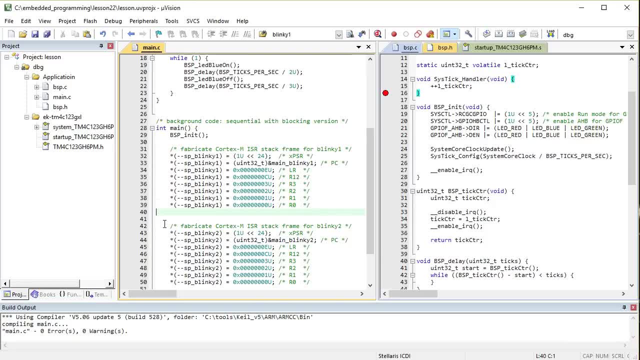 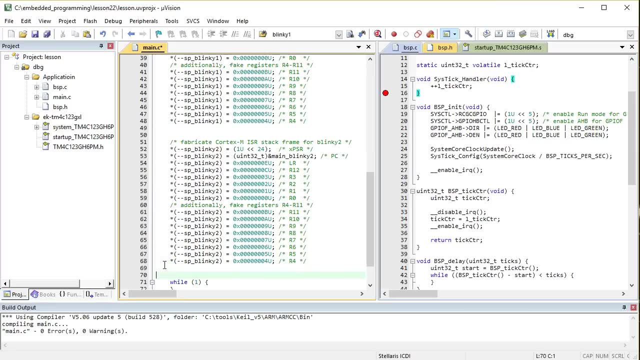 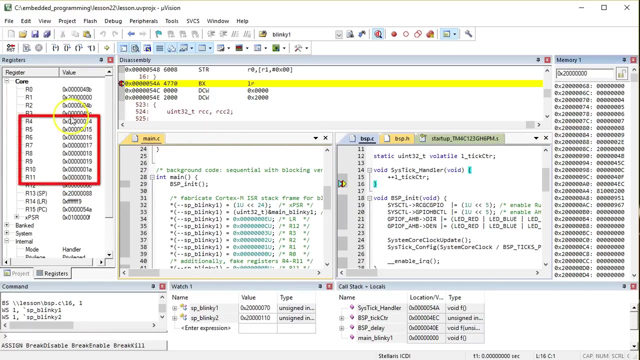 you've been doing so far. First, you need to append the additional registers to the fabricated stack frame for all your threads. Second, when saving the current thread context, you need to save the additional eight CPU registers, R11 down to R4..